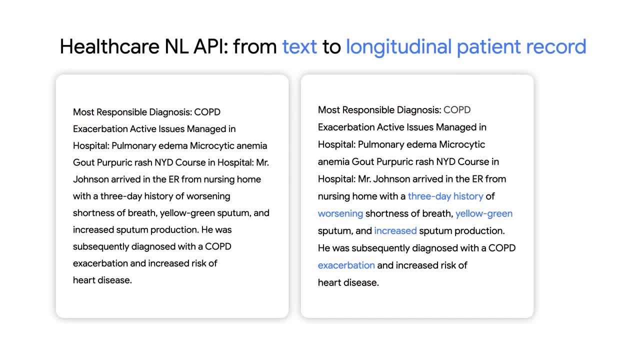 Another way of thinking about NLP is that it can extract critical clinical information, like medications, medical conditions, as well as understand contexts like negation, such as this patient does not have diabetes. It also understands temporality, such as This patient will start chemotherapy tomorrow, and even infer there are relationships between things such as side effects or medication dosage. 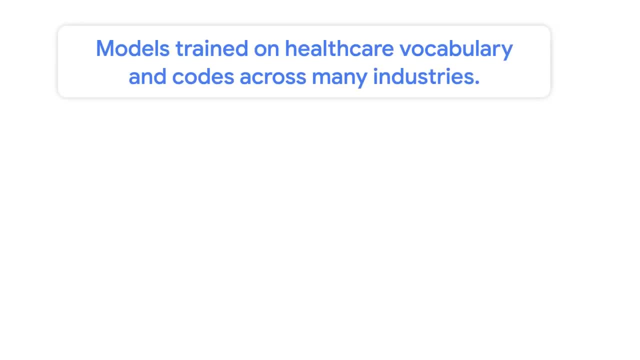 And what's most notable is we have a long list of ontologies the natural language models are trained with. Two notable ones are the ICD, which is used to code and classify morbidity data from inpatient and outpatient records, physician offices and most national center for health statistics services. 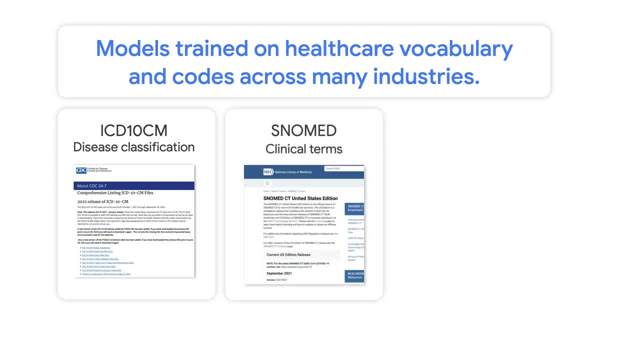 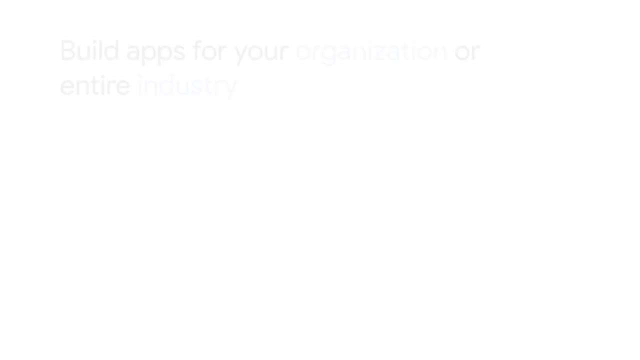 There's also SNOMED clinical terms, which provides core terminology of electronic health records. The models also include US official codes for insurance procedures and RX norm, which contains a list of all medications available. Technical practitioners can leverage healthcare NLP to build apps for their own organization or for their entire industry, such as enabling precise search and discoverability across patient populations. 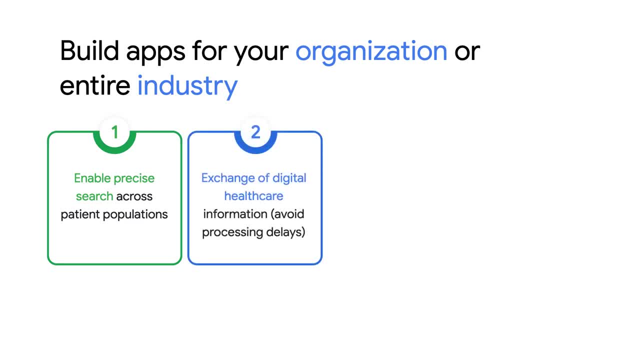 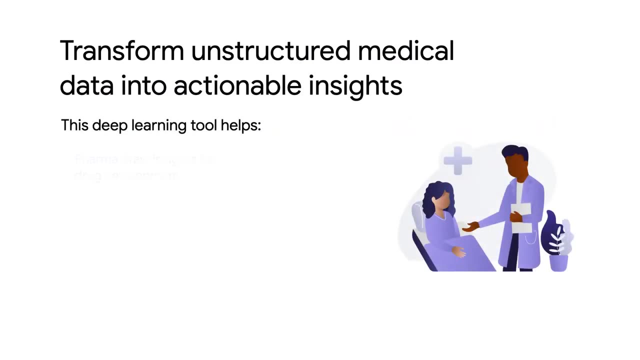 Enable accessibility to medical applications, exchange of digital healthcare information and avoid processing delays, establish and maintain regulatory compliance or automate administrative workflows, such as identifying and eliminating errors that require corrective activities. Anyone who has science-based texts around research or clinical data can get value from our Healthcare NLP API. Here are a few sectors that can benefit. 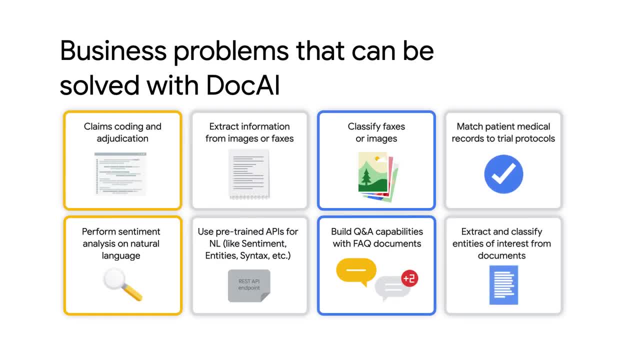 to name a few. In telehealth, you now have off-the-shelf support for exchanging medical knowledge captured in written form and can extract structured knowledge from text and make it available for digital services such as chatbots, call centers, clinical decision support systems. 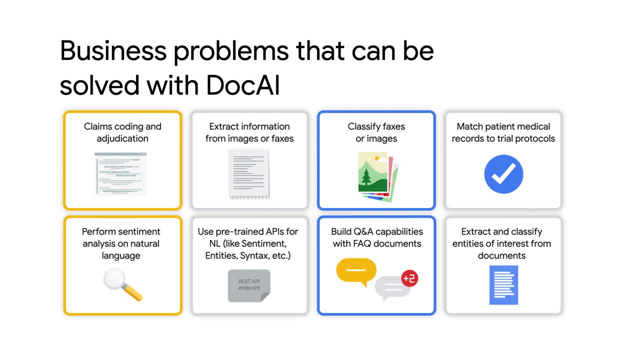 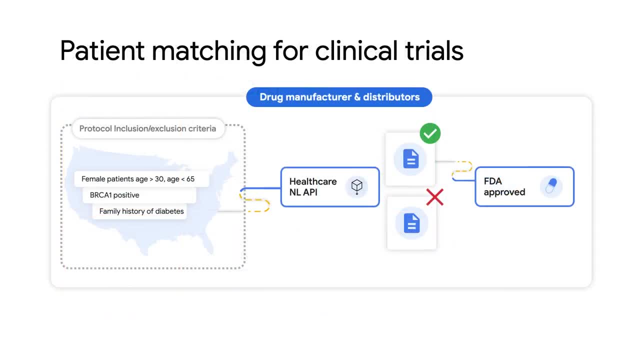 This also frees up time by triaging patient calls and resolving cases that do not require the intervention of a clinical professional. Pharmaceutical researchers are also enabled, via NLP, to provide clinical support for their patients, For example, if you have a patient discovery interface for population health and R&D applications since papers and clinical trial. 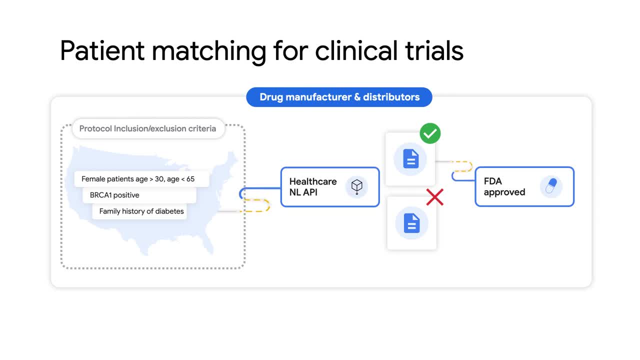 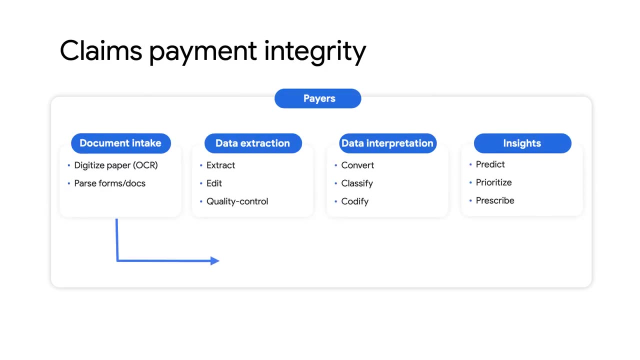 documentation can be surfaced to match patients or find novel treatments. Those managing clinical trials can both increase their number of participants as well as process the high volume of feedback and decrease time to government approval. Users who manage billing, especially in insurance companies, can have even better integration with claims payment or automate. 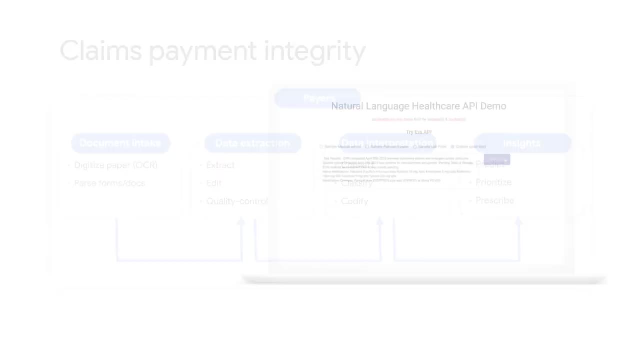 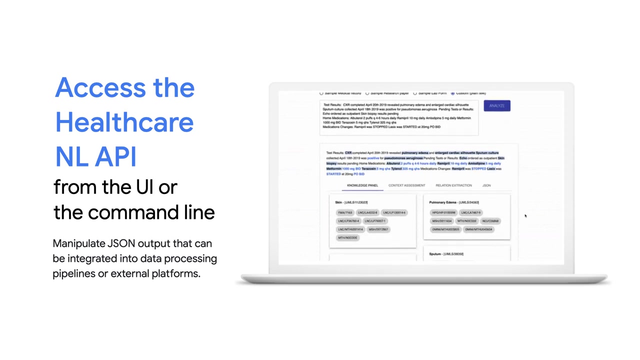 billing and coding for insurance. You can enable the Healthcare NLP from your Google Cloud Projects UI or via the command line. If you do not have a project, there's a link in the description, along with other helpful resources, And once you have set up permissions, you can begin using its. 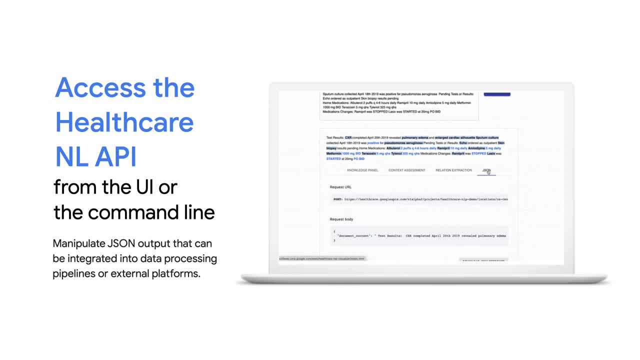 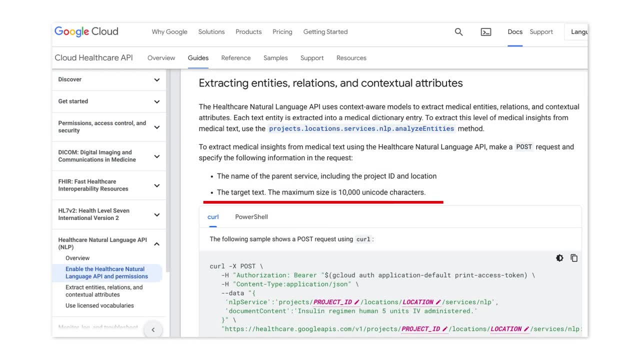 context-aware models to extract medical entities, relations and contextual attributes. Each text entity is extracted into a medical dictionary entry. To extract medical texts: make a post request and specify the following information in the request: First, the name of the parent service. 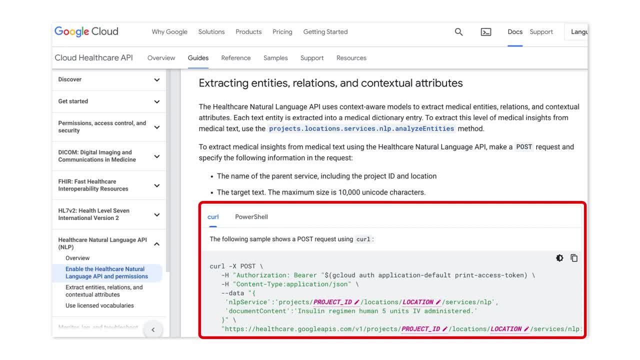 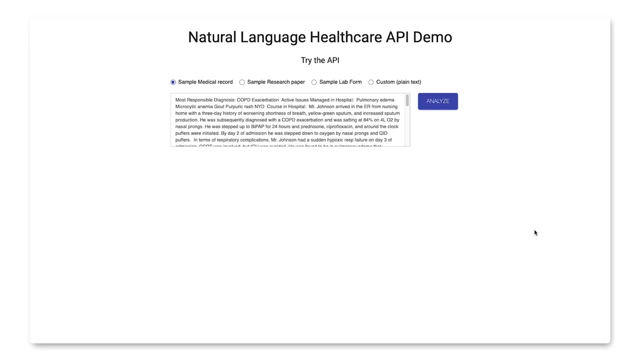 including the project ID and location. Also the target text. The maximum size is 10,000 Unicode characters. at this time. Let's quickly show you how you can leverage the Natural Language Healthcare API. We built a demo application with a JavaScript front-end to visually understand the output of. 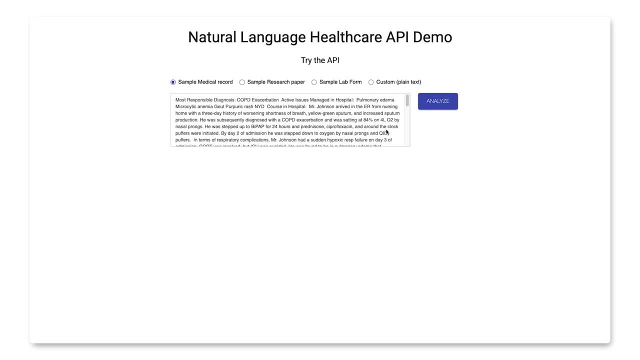 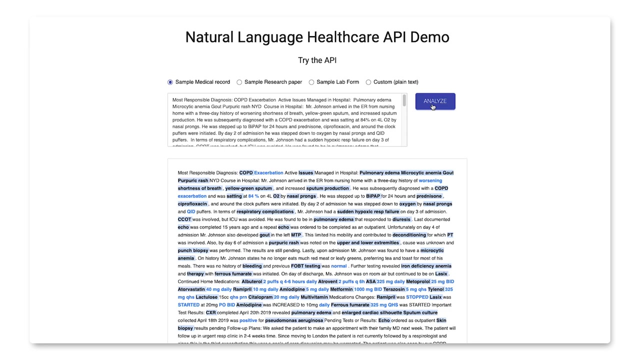 the Healthcare NLP API. Let's test out the application. We test out the sample medical record for a hospital patient. We send over the sample medical text to the API on the back end and we render the JSON response in this web app. 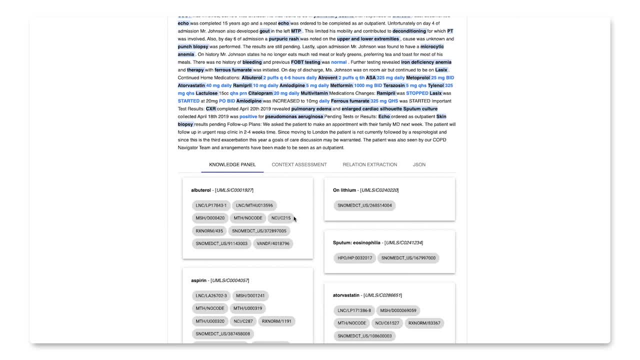 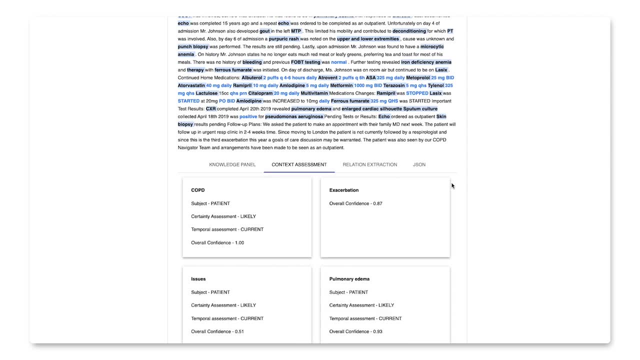 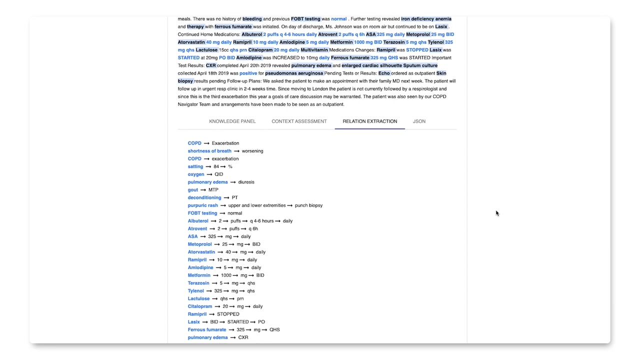 In the first panel down here we can see the various entities extracted and their corresponding medical code. Next we can see their diagnoses with their corresponding confidence scores. Now, looking at the relationships between the entities, we can actually group together important attributes. For example, take a look at how long and how much of these medications. are taken or were prescribed. There are so many possibilities when using healthcare and health care. Thank you for joining and making this video. If you enjoyed this video and would like to see more, please subscribe and click the bell button. We'd love to hear from you.